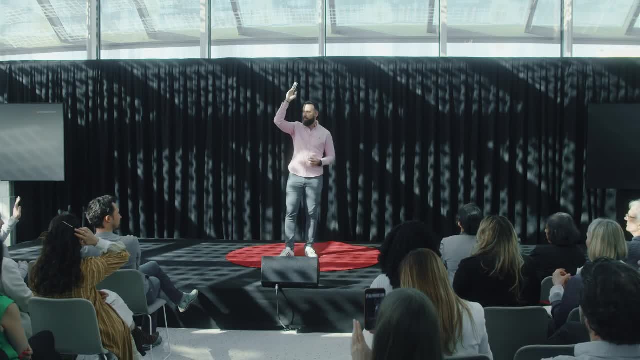 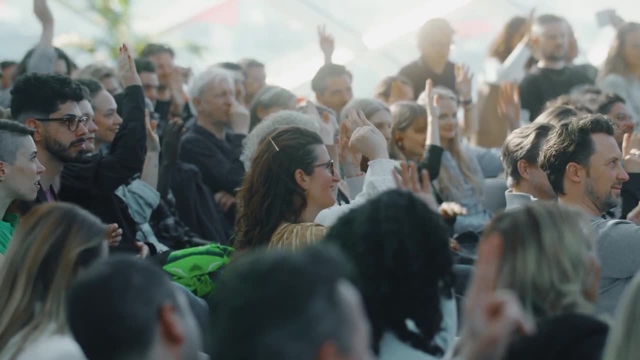 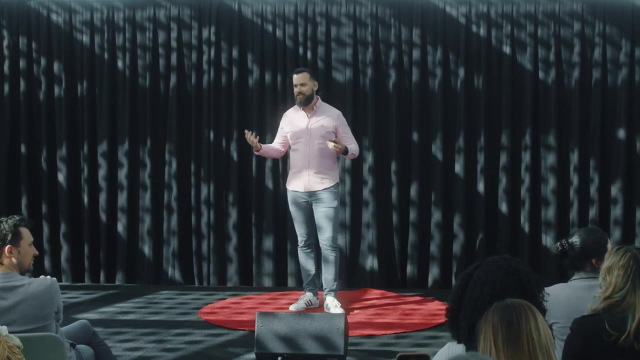 Now please keep your hand up, Hold it up. Hold it up Now. keep it up, if you would leave a teenager unsupervised with your card. See, your fears are justified. To the brave fruit, congratulations. But your fears are justified. Teens just don't have the necessary. 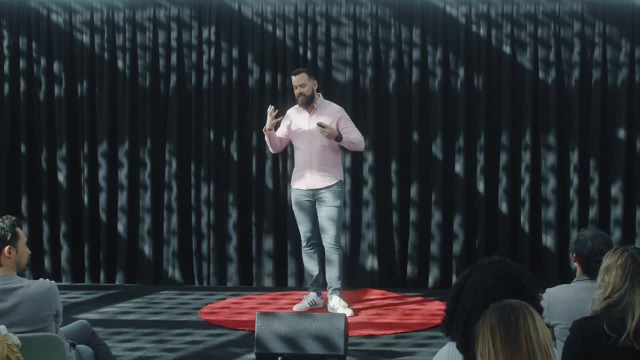 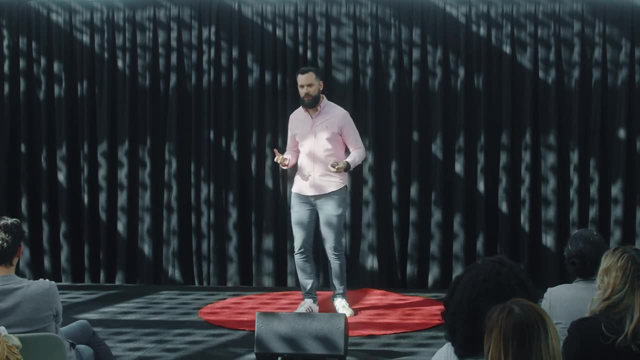 money skills. It's not taught at home, It's not taught at schools, actually. And you go into a school and you hear stuff like mitochondria is the powerhouse of the brain. You go into the cell. You don't hear the government is going to take part of your salary as taxes. 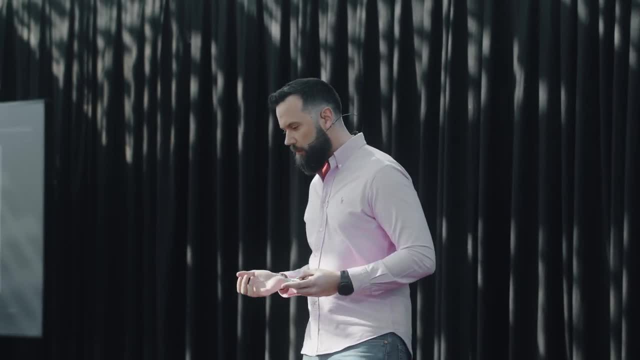 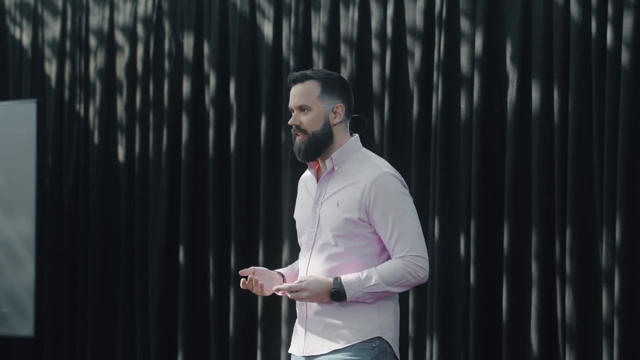 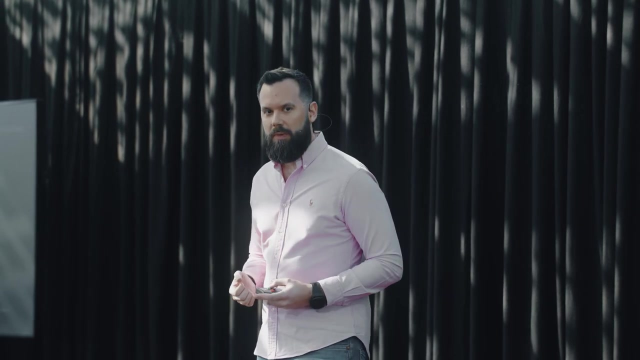 It's just not taught. They don't teach them budgeting or savings. And essentially, when I say it's taught at home, what happens is I walk up to my dad and I say: dad, how do I lower my credit card bill Like it's huge Dad? dad, please help me, I'm losing all of 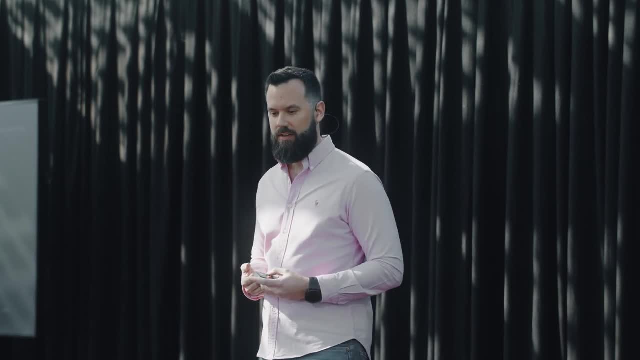 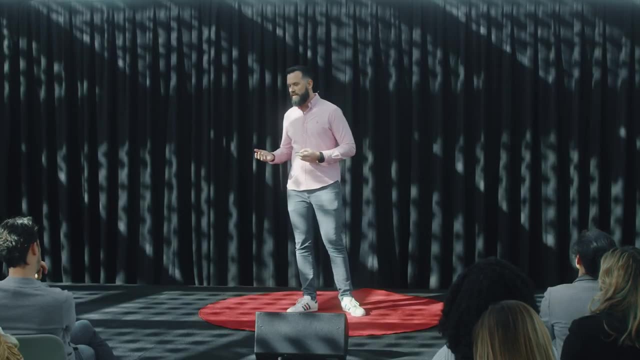 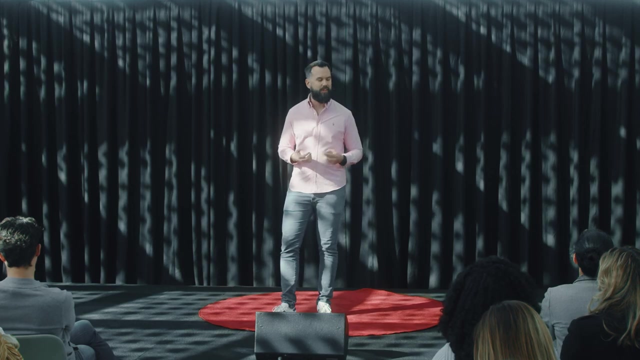 my money on crypto. Dad. dad, teach me this stuff. He has good answers to a lot of them. But stuff like dad, should I hodl my board apes collection to the moon and then sell it on OpenSea for ETH and then pancake swap that? 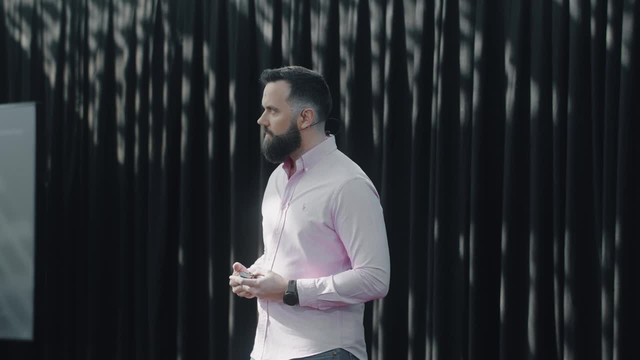 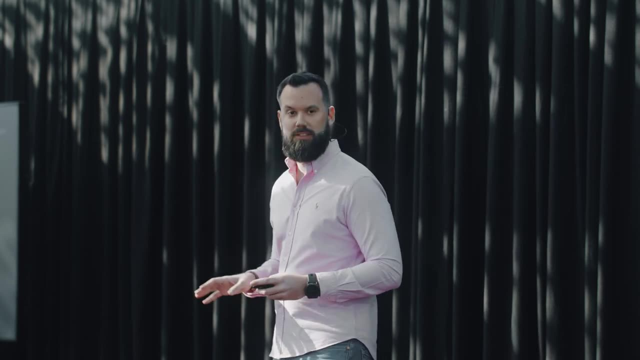 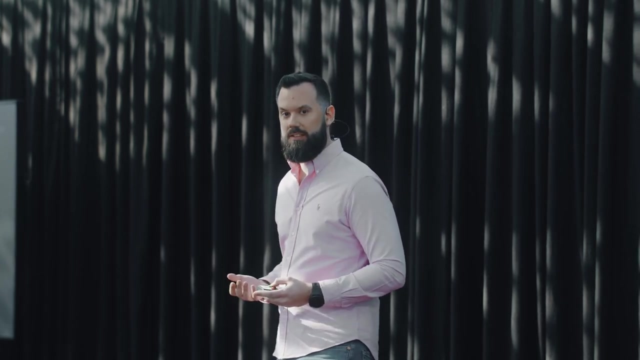 into USDT for lower fees. Yeah, that just doesn't work. And for most of us here, what I just said is complete and utter nonsense, And it's okay if you feel lost, But it really is the jargon that teens are using these days. 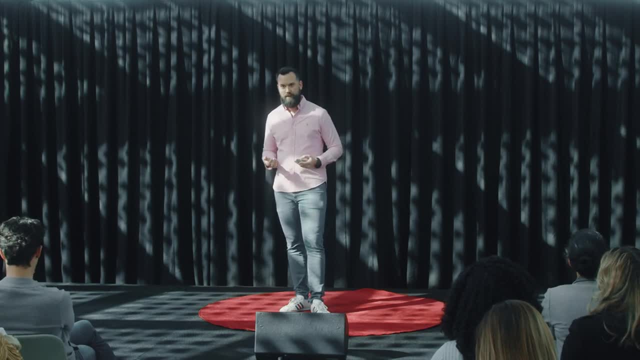 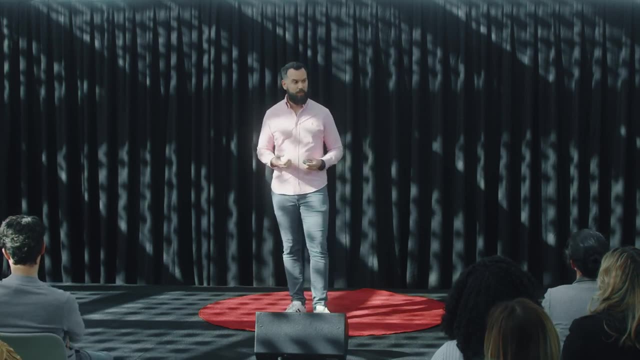 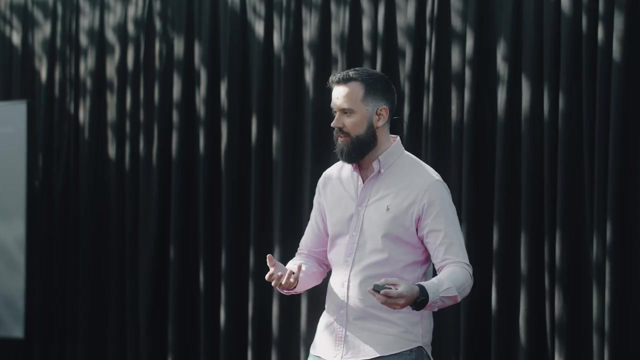 It's normal, It's the new mainstream. We built NickyCard to help parents answer some of these tough questions. Parents talk to us and they told us my teens do not understand the value of money. They think it comes out of thin air. They said we struggle to motivate. 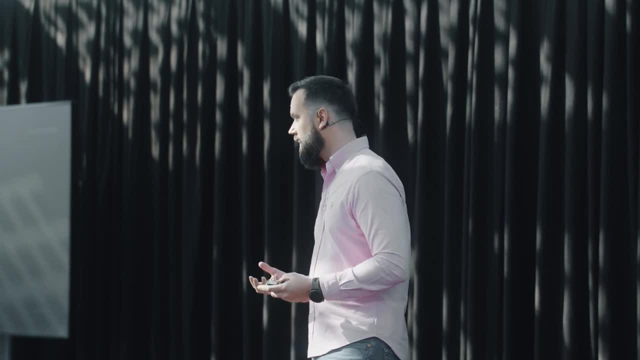